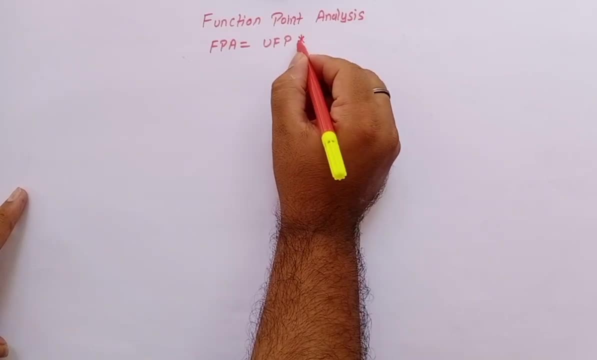 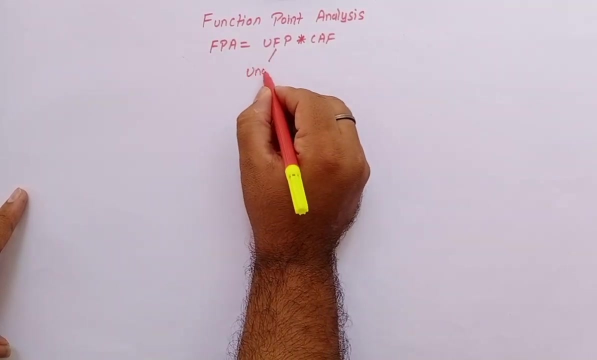 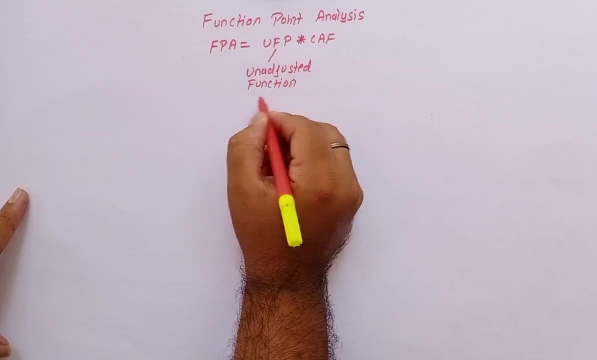 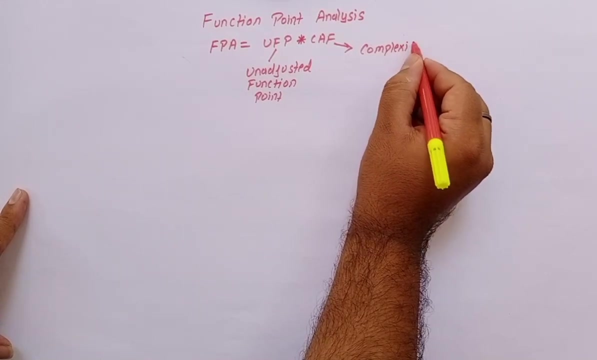 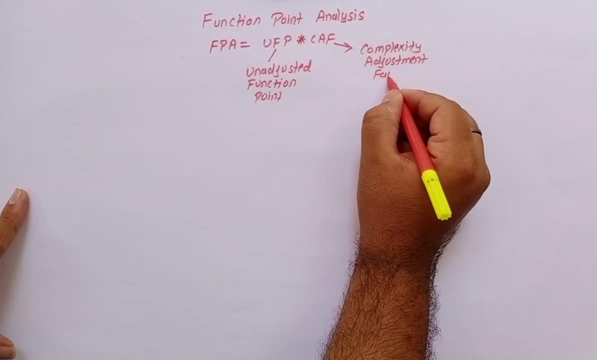 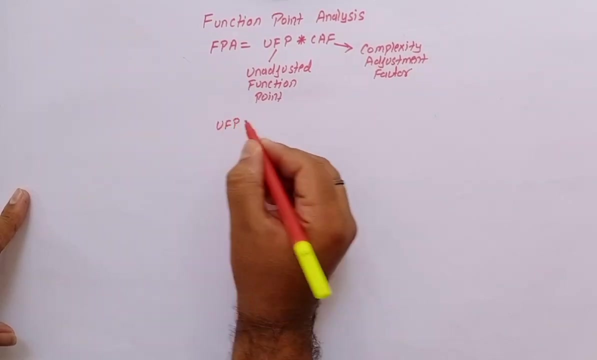 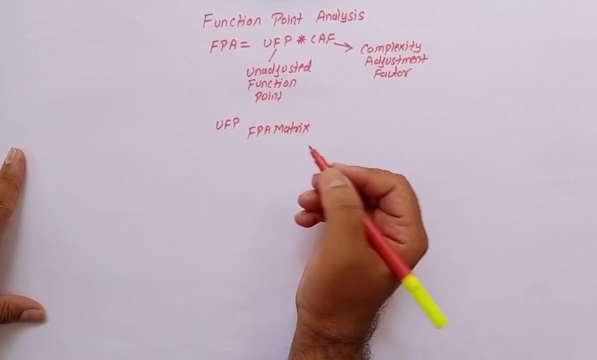 FPA is equals to UFP into CAF, where UFP stands for unadjusted function point complexity adjustment factor. Now how to calculate UFP? In order to calculate the UFP, we have to first understand the function point analysis matrix. So FPA matrix In FPA matrix. 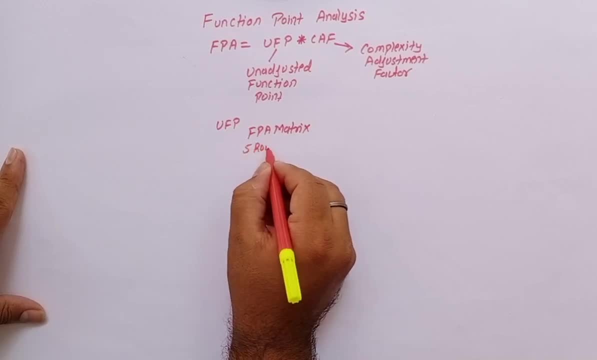 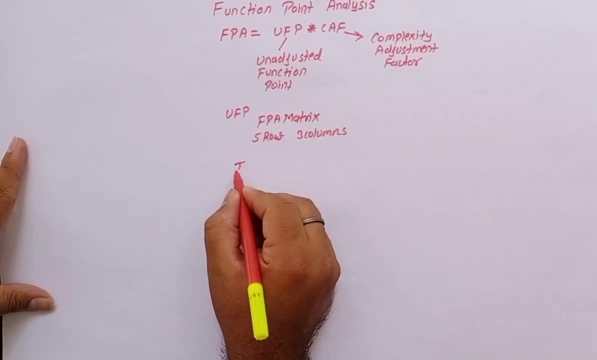 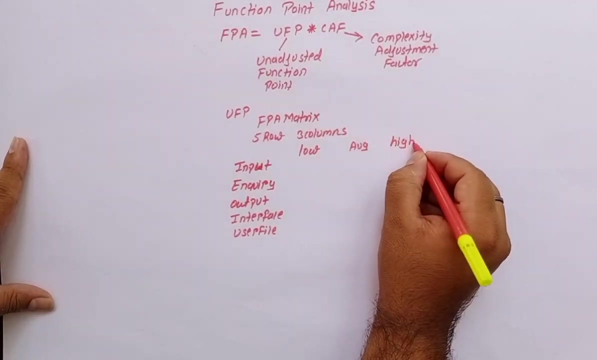 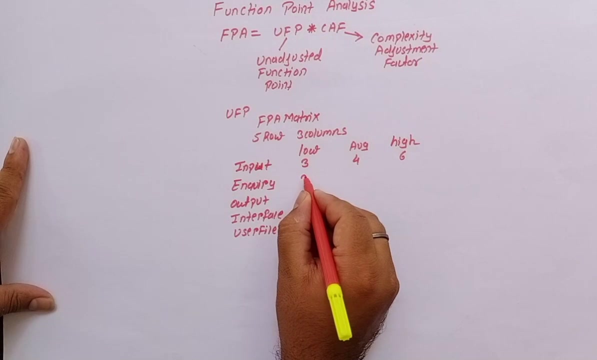 we are having a 5 row and 3 columns. So row represents input, enquiry, output interface and user file, And column has value low, average high For input value is 3,4,6.. For enquiry: 3,4,6.. 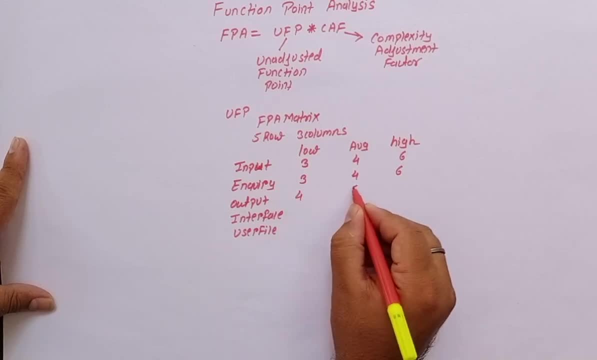 For output value is 4,5,7.. For interface: 5,7,10.. For user file: 7,10,15.. This matrix is known as FPA matrix And this values are called weight adjustment factor. Now, formula for calculating UFP is: UFP is equals to summation. 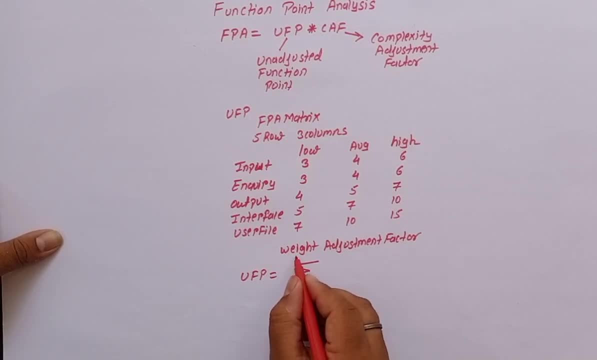 period. I value is equal to 1, J value is equal to 1 till I value is equal to 5, J value is equal to 3, W, J, C, J, where W is equals to wait adjustment and C is equals to count. 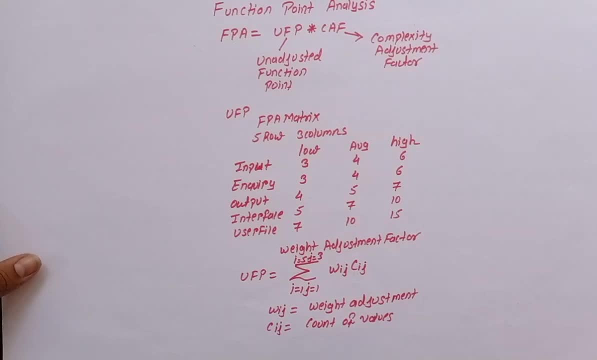 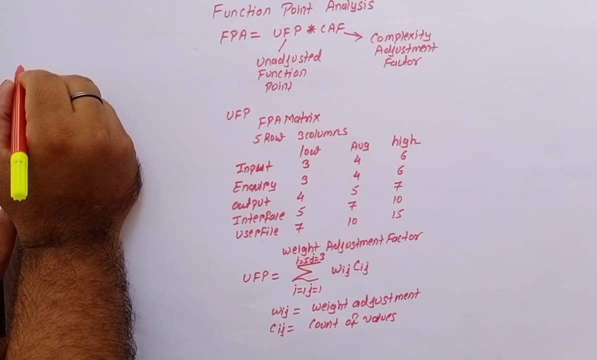 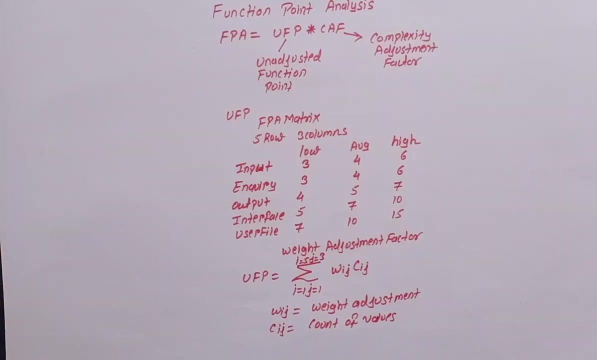 values now. now let's see how to calculate a CAF. but before calculating a CAF, let's see functional point. analysis makes the use of 14 important characteristics of a software. now, while calculating a CAF, we have to consider all these 14 factors, or 14 software characteristic, and their degree of. 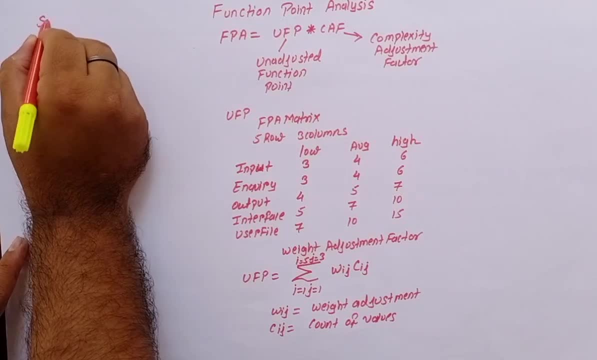 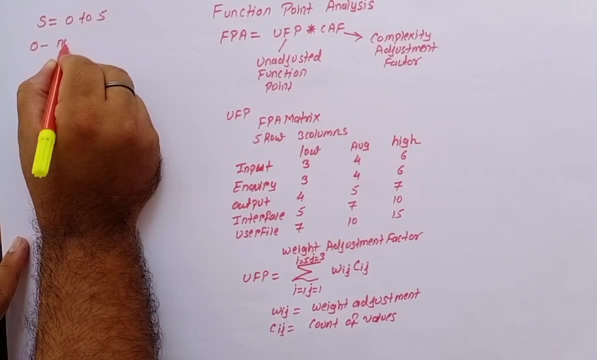 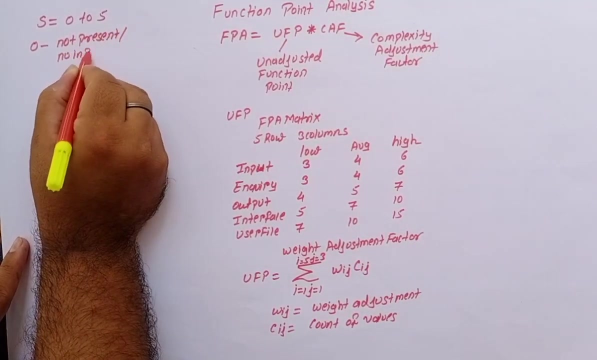 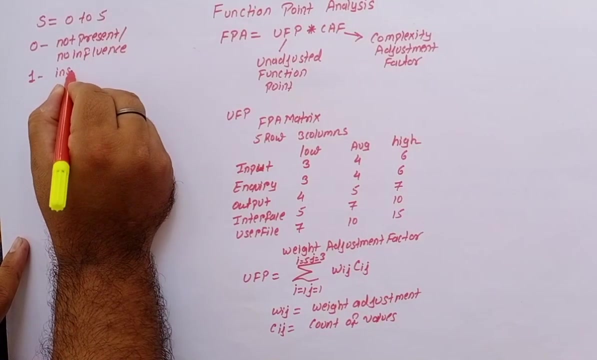 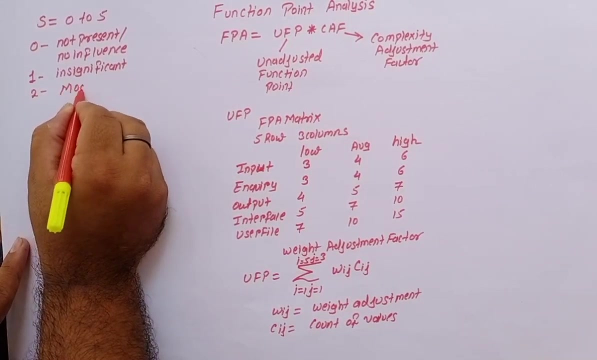 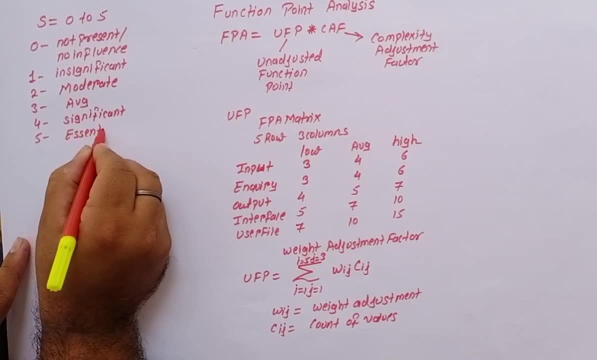 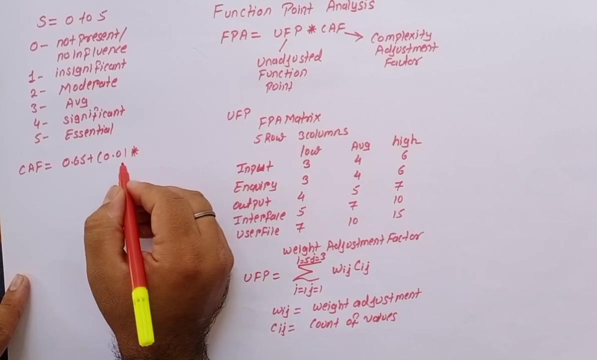 indicates essential. now the formula for CAF is 0.65 plus 0.01 into, since we are considering 14 important characteristics or features of a software. so we are going to multiply with 14 into the value of degree of significance. that is s. now the maximum value of CAF can be 0.65 to 0.01 into 14. 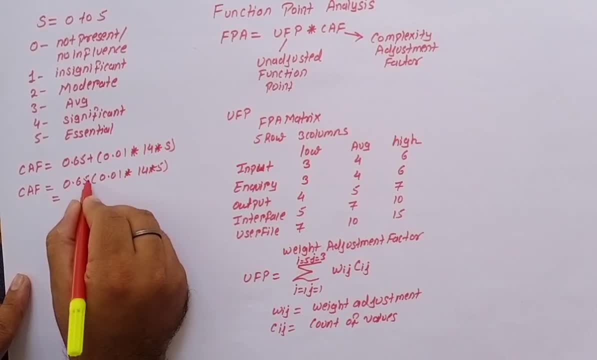 into 5, that is 0.65 plus 0.01. into 70, that is 0.65 plus 0.7, that is 1.35. so maximum value of CAF cannot be more than 1.35 and the minimum value of CAF can be. 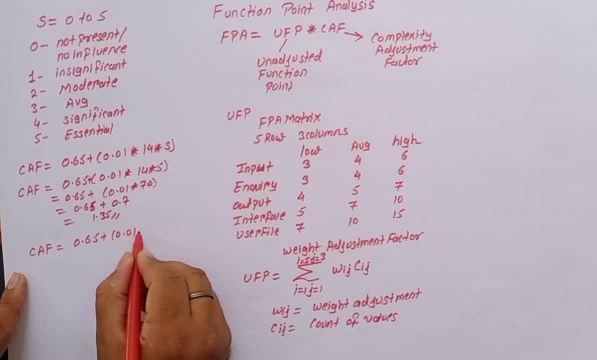 0.65 plus 0.01 into 4.35, into 0. so the minimum value of CAF is 0.65. now we know that. how to calculate UFP, how to calculate CAF. after calculating UFP and CAF, we are in a 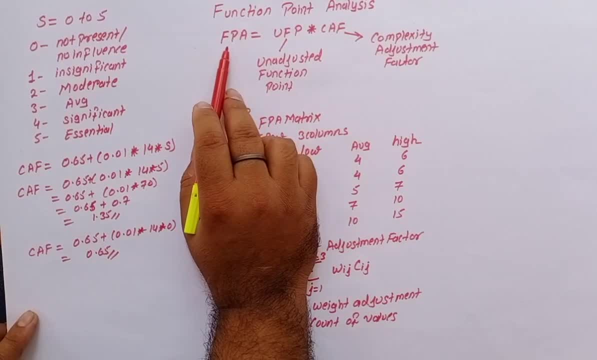 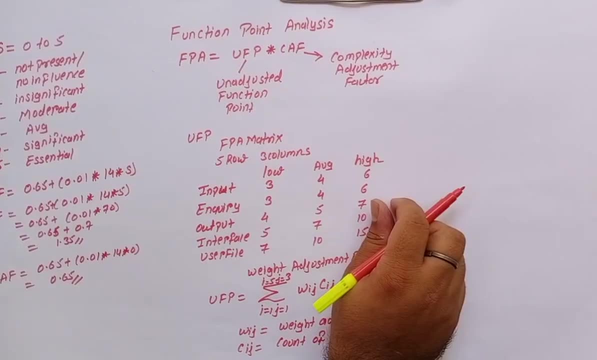 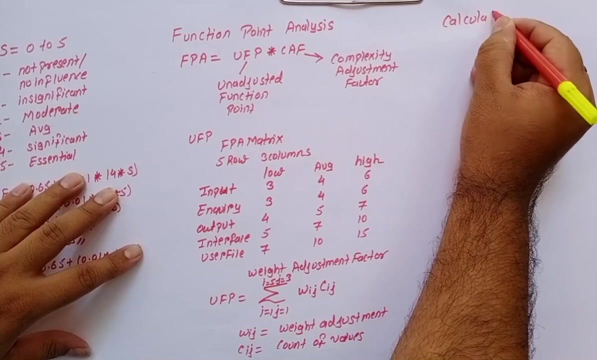 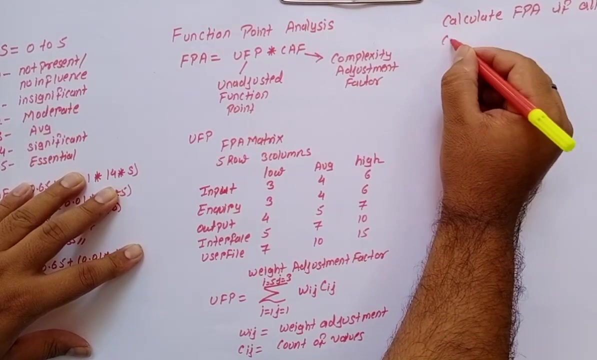 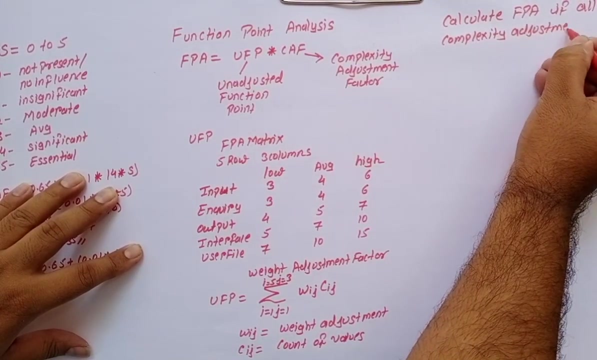 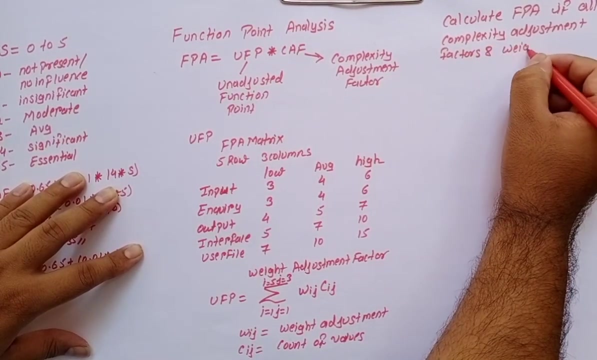 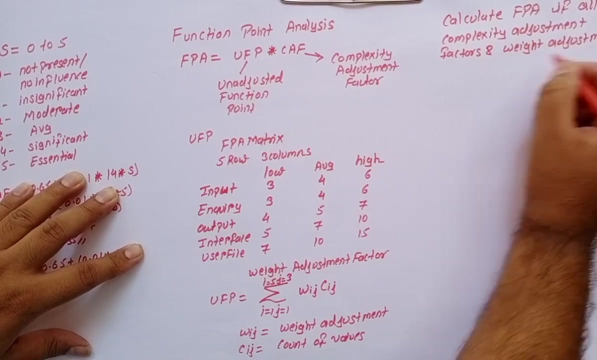 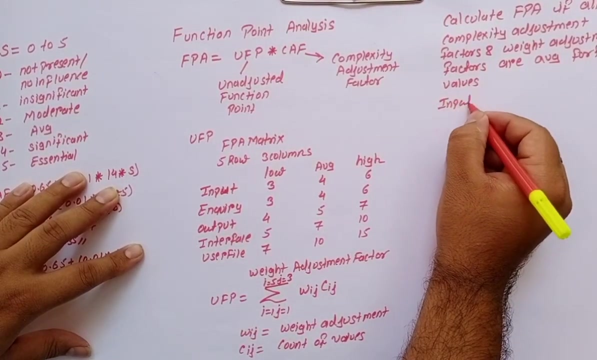 position to calculate the function point analysis, which is equals to FPA, is equals to UFP into CAF. let's solve one numerical question on function point analysis: calculate FPA. if all complexity, adjustment factors and weight adjustment factor are average for following values: input is equals to 10, output is equals to 30. 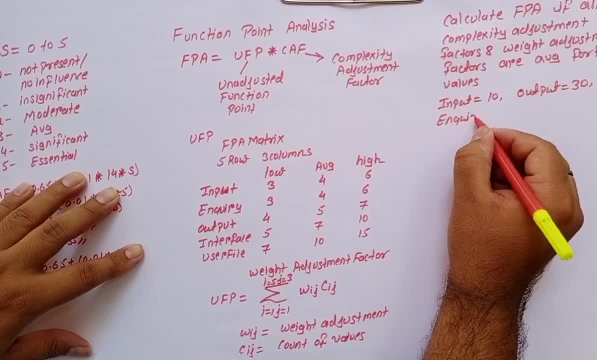 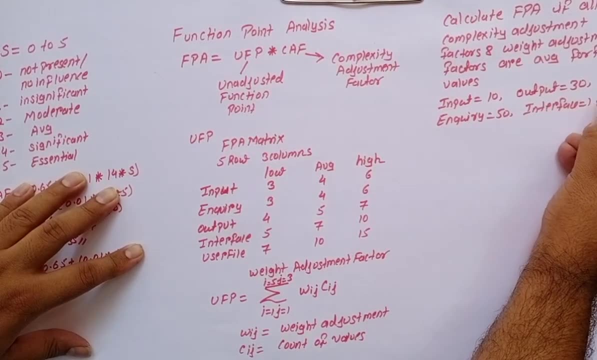 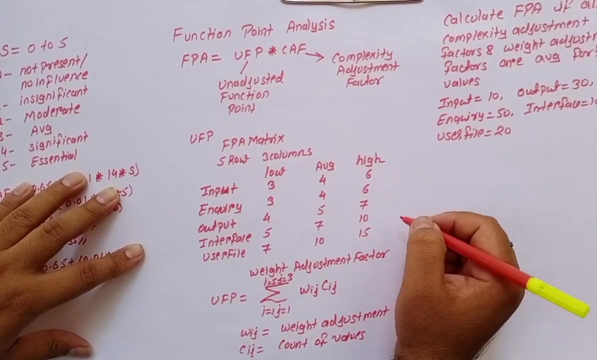 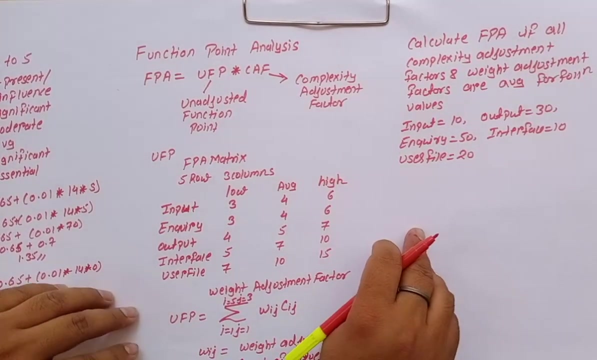 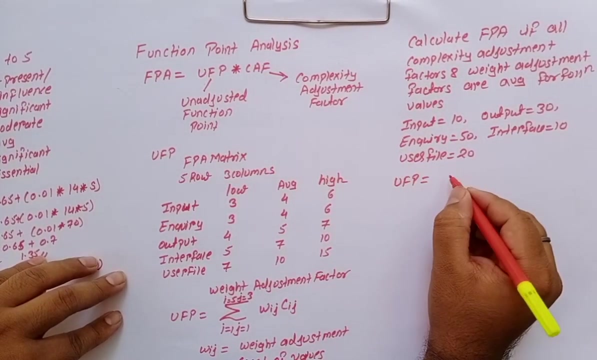 inquiry is equals to 50, interface is equals to 10 and user file is equals to 20. so first we are going to calculate UFP. so for calculating UFP, we all know that formula is: I equals to 1, J equals to 1, I equals to 5, J equals. 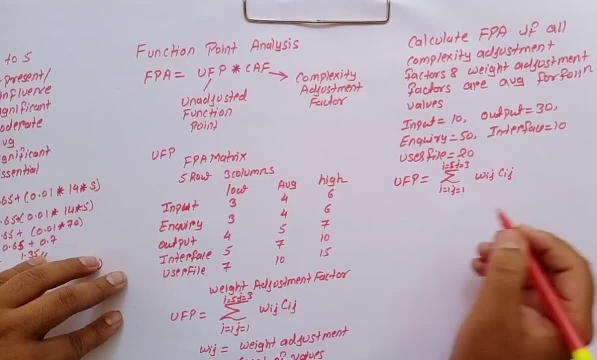 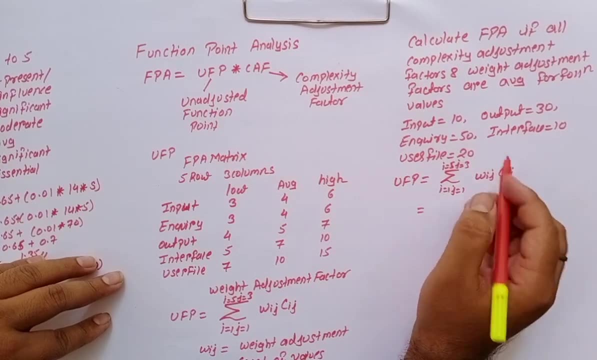 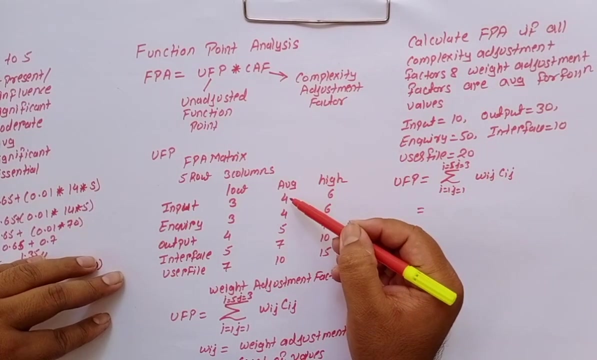 to 3 W of IJ into C of IJ, where W of IJ is weight adjustment factor and C of IJ is a count of number, since in a given problem they have mentioned that weight adjustment factor are average. so we have to consider this column now. the count: 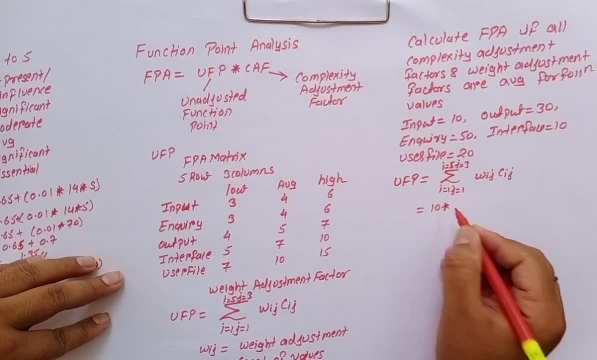 of input is 10 and the weight adjustment factor is average, so 10 into 4, and query is 50, so 50 into 4. output is 30, so 30 into 5. plus interface is 10, so 10 into 7. user file is 20, so 20 into 10, so we will get 40 plus 200 plus 150 plus 70.